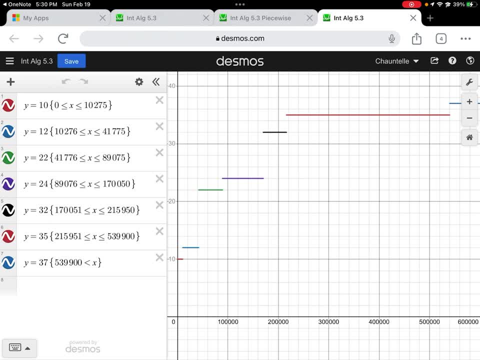 So if you're going to graph each one of those notice I have: y equals 10 when x is between 0 and $10,275 and so on, And I had to adjust all of my axes so that these would all show. And you do that by going into the. 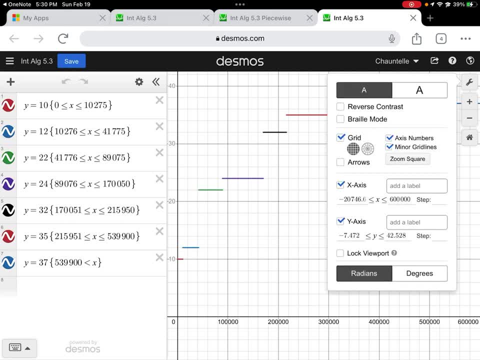 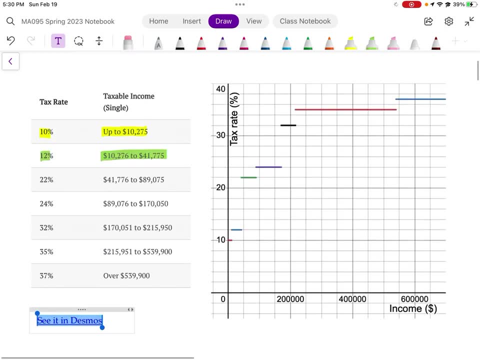 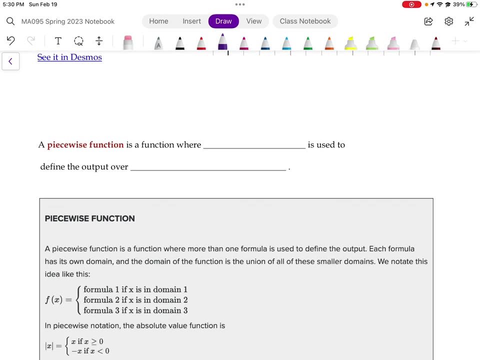 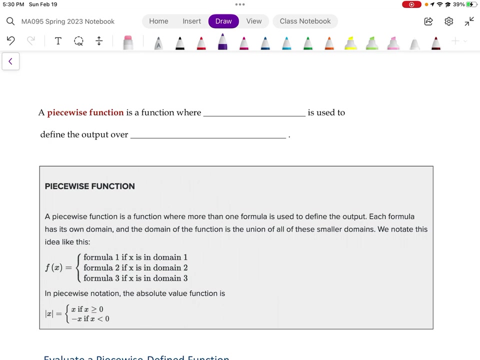 tool button. So I changed my x-axis and I changed my y-axis. All right, so, coming back here, you'll need to know when you go into Desmos how to, how to change the domain and range. Okay, so a piecewise function is a function where more than one equation, more than one. 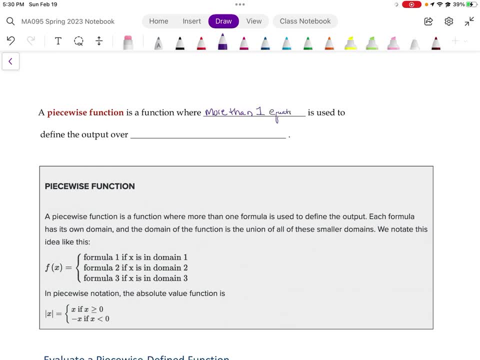 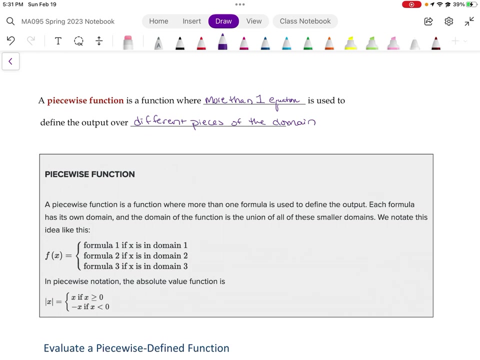 oh, I didn't leave enough room, did I? Equation is used to define the output over different pieces of the domain. different pieces, Okay. so a piecewise function is defined right here below. More than one function is used to define the output. 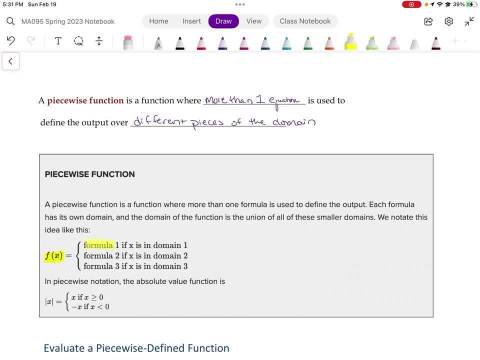 Okay, so in other words, f of x equals this first equation if x is in the first domain, This other equation, formula two, if x is in another domain and this other equation if x is in another domain. So if x is in another domain, then this other equation, formula two, if x is in another domain. 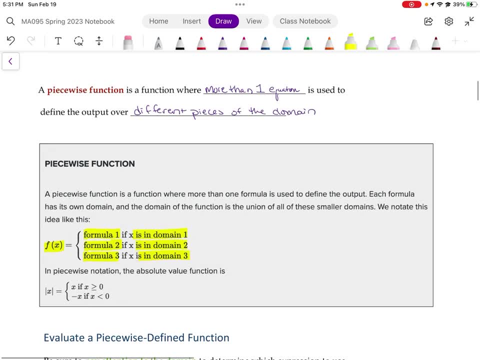 then this other equation, formula three: if x is in another domain, then this other equation is in the third domain, And you can go on and on like that if you'd like. It can have as many as it needs. Okay, so an example of that is an absolute value function. 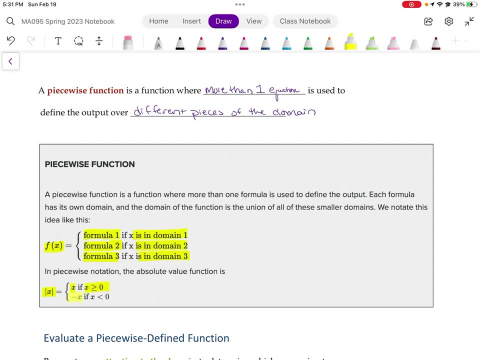 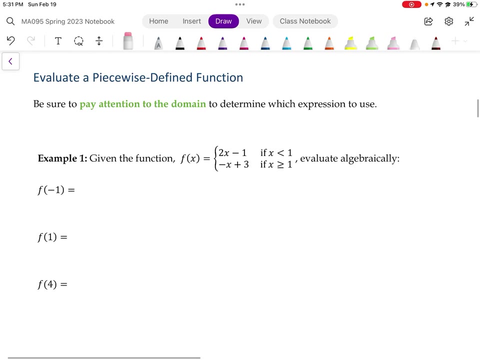 So absolute value is x when x is equal 0, and it's the opposite of x if x is less than 0.. All right, So, continuing on from there, let's look at evaluating a piecewise defined function. So be sure to pay attention to the domain. 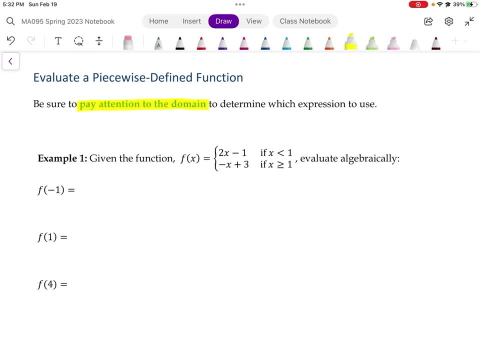 I put it in green there. I really want you to pay attention to that. Pay attention to the domain. Did you do that? No, determine which expression to use. Okay, so we've got here that f of x equals 2x minus 1. 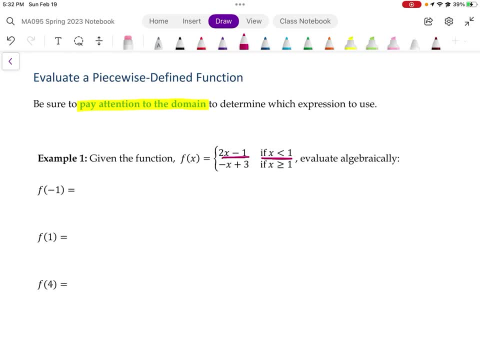 when x is less than 1.. And it equals this other equation if x is greater than or equal to 1.. Okay, so that's what we mean by pay attention to the domain. All right. so we're going to say: all right, what is f of negative 1? f of negative 1.. So we need to go look for where is f. 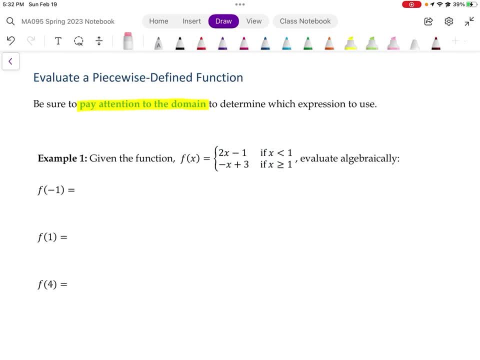 where is x? I'm sorry, less than 1, because that is the input, right? So remember, when we look at f of negative 1, this is the input, which is x. So you need to go look where x is less than 1.. x is less than 1, right there. So f of negative 1 is going to be evaluated with 2x. 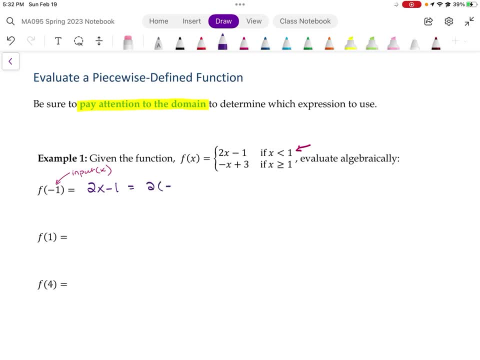 minus 1.. That's the one we're going to use. Well, x is negative 1 in this case. So 2 times negative, 1 minus 1 is is going to be negative 2 minus 1, which is negative 3.. Okay, so that is going to be the. 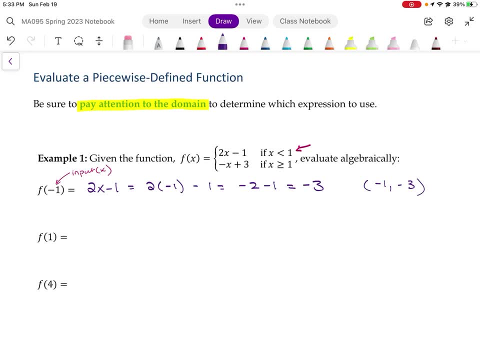 point. negative 1, negative 3.. All right, so f of 1, which one are we going to use? So you've got to go look and see which one we're going to use. Is it going to be? is 1 less than 1, or is it? 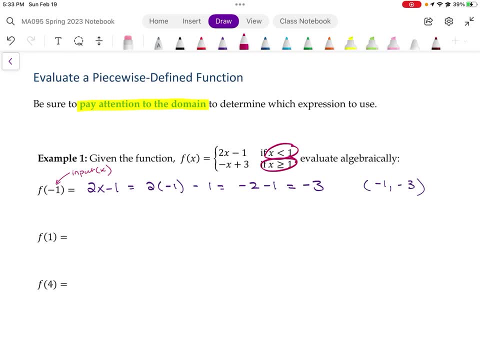 greater than or equal to 1?. Well then, it's great, It's equal to right. So you're going to use the second one. So, in this case, we're going to use the second one. All right, so we've got. 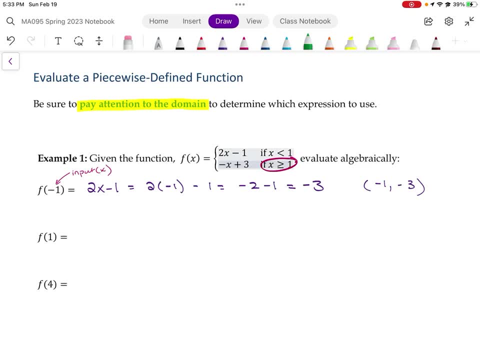 I'll use a different color, because each of these you've got the equation negative x plus 3.. That's the one we're going to use. Okay, so that's this equation here. So we've got negative. our value for x is 1, just plugging it in right there. 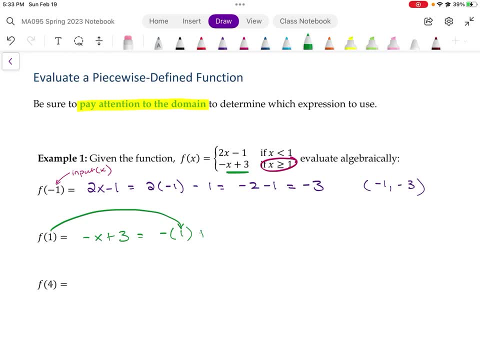 plus 3.. So negative 1 plus 3 is 2.. So we have the point here: 1,, 2, and that's on the other line. All right now. the last one is f of 4.. What is 4?? Which domain is it in? Is it in the first domain or the second domain? 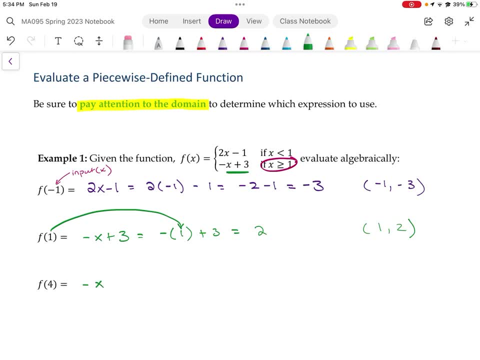 Well, it is greater than 1, so we're going to use the negative x plus 3, the green one. Okay, so I'm going to. I guess I'm color coding these, just decided as I'm working here. The top one is: 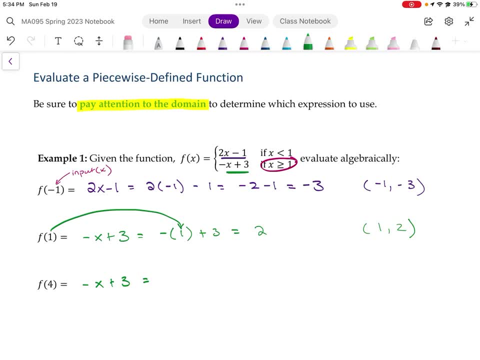 the purple one, the bottom one is the green one, and the green one is used for the second two. Okay, so you just have to pay attention. So negative 4 is our number plus 3, negative 4 plus 3 is negative 1.. So this point, the input, is 4,. 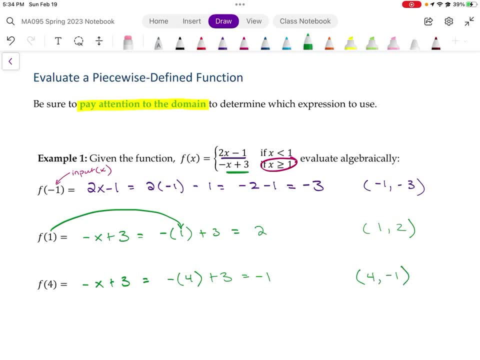 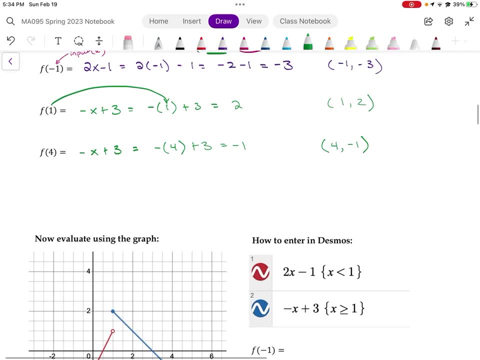 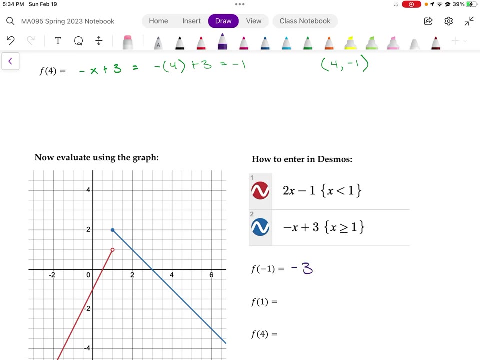 the output is negative 1.. So there's our point 4, negative 1.. All right, so now let's check using the graph. All right, so we just had. let me rewrite these: f of negative 1 was our purple one, that was negative 3.. f of 1 was 2,. 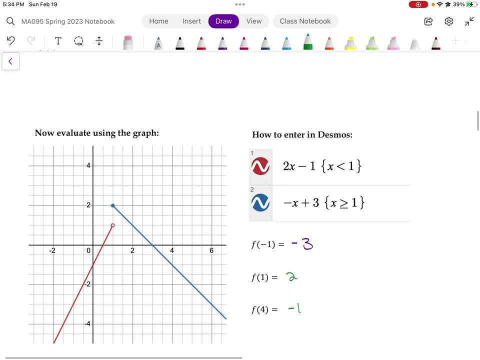 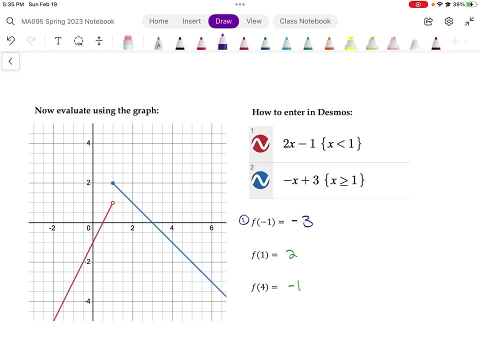 and f of 4 was negative 1.. So let's take a moment, pause the video and see if that is true on the graph. So let's go look, So point. we'll call this one point, one F of negative one. 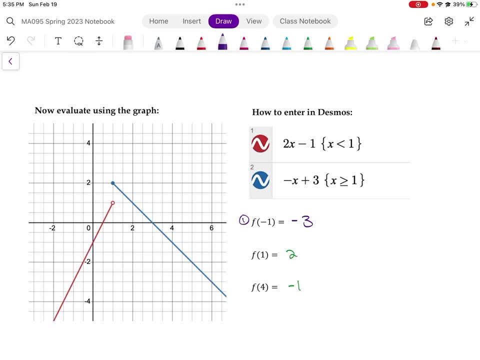 So negative one is here to the left of zero. Go down and I get F of negative one lands right here And that, sure enough, is negative three. Be careful reading this because there's extra lines in there for point five. All right, the second one is: F of one equals two. 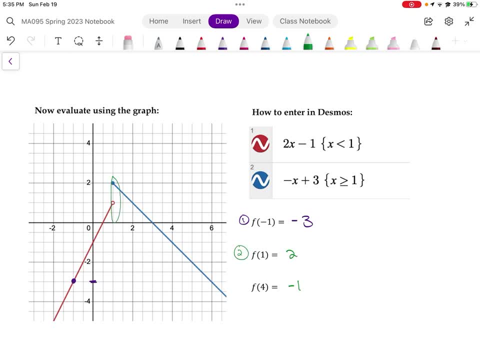 So let's go over to one And let's see. we've got two choices here. Which one is it going to be? Well, the open circle means it's not there. The closed circle means it's right there. That's where it is. 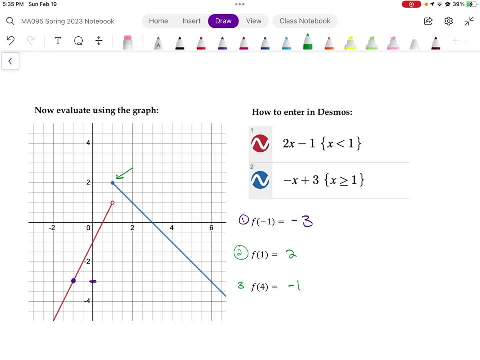 So it does equal two. All right, now try. so that is point two. right there, Let's label point one as well. Forgot to do that. There's point one. So point three, where is that? F of four is negative one. 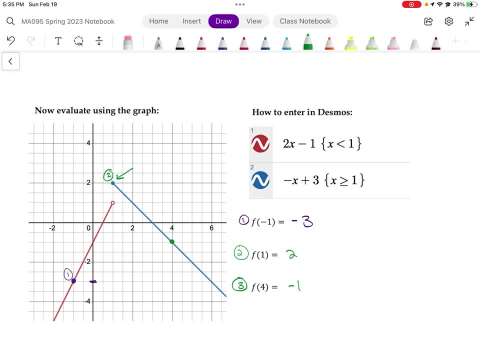 F of four is negative one right here, And sure enough, that is correct. So that is point Point three. Okay, so I just checked using the graph. Now I wanted to show you also how to enter it into Desmos, And this is how we do it, right here. 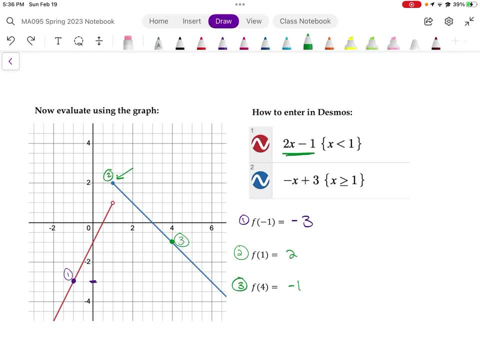 So you're going to say F of X equals, and here's your equation. I'll stick with my color scheme. Here's your equation. right here, When X is less than one, you use these curved brackets. Okay, All right, And you're going to use inequality notation. 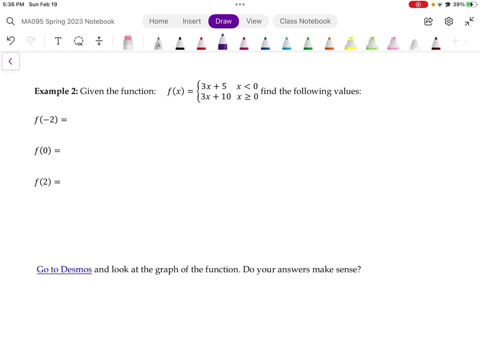 All right, so moving on, Pause the video. Let's see what you can do with that. Okay, so hopefully you gave it a try. So we're going to have this one be purple and this one be green, like before. If X is less than zero, we're going to use the first one. 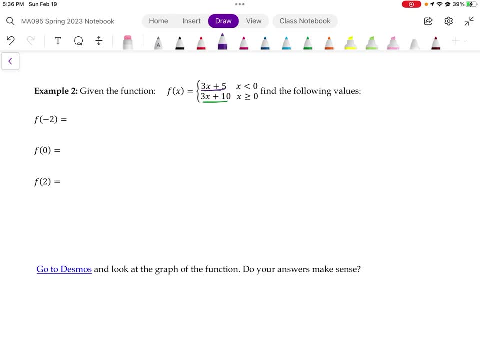 If X is greater than or equal to zero, we're going to use the second one. So F of two, No, sorry, negative two. F of negative two is our first one, So it's less than zero, So we're going to use the first equation, the purple one. 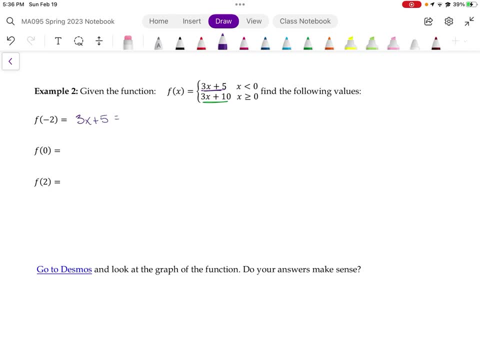 So we've got three: X plus five is the one we will be using. So we've got three times negative. two plus five is going to be negative six plus five, which is negative one. So our point now is negative two, negative one. 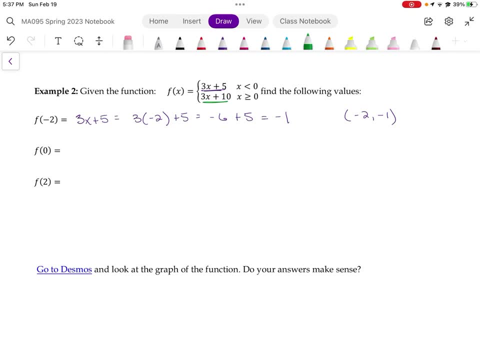 All right. next, F of zero is greater than or equal to zero, So it's equal to zero. So we're going to use the second one, That is three X plus ten. So we've got three times zero plus ten is zero plus ten, which is ten. 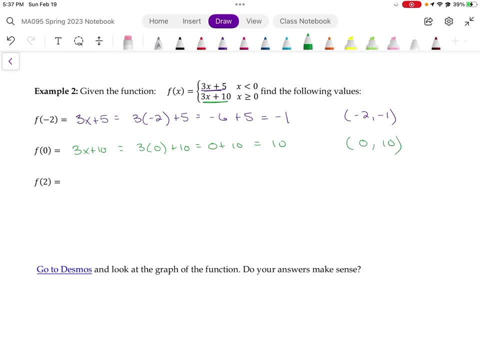 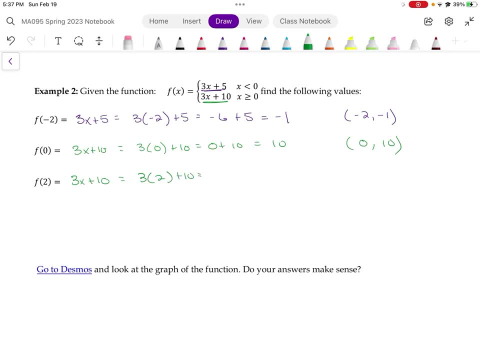 And that is three times two plus ten, which is six plus ten, which is sixteen. So we've got two. sixteen is our point. Now you can go to Desmos and check that on the graph of the function and make sure your answers make sense. 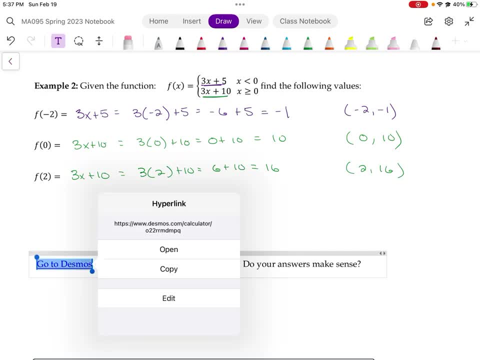 Okay, so I will go there so you can see it. I'm going to open that Now. you have to be in text mode to be able to do this. When you're in drawing mode you can't get those hyperlinks to work. 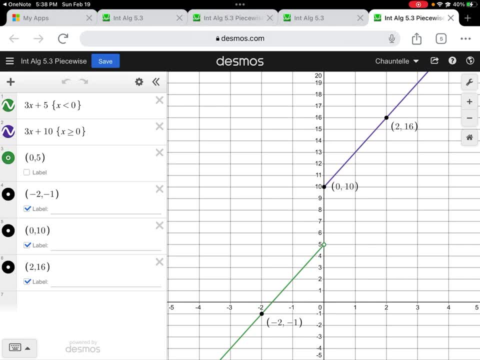 All right, so there's all our points, the three points. Notice- I put an open circle just so you could see it- at zero five, because the green one is less than, not less than or equal to The purple one is greater than or equal to zero. 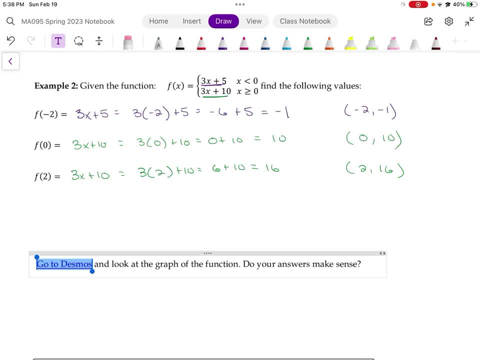 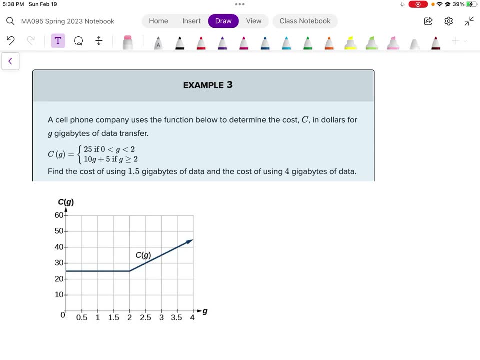 Okay, so, going back where we were, move back down. Now we're going to look at something. This is a real-world problem. A cell phone company uses this function below to determine the cost for gigabytes of data transfer. So if you use between zero and two gigabytes, of course not equal to zero. 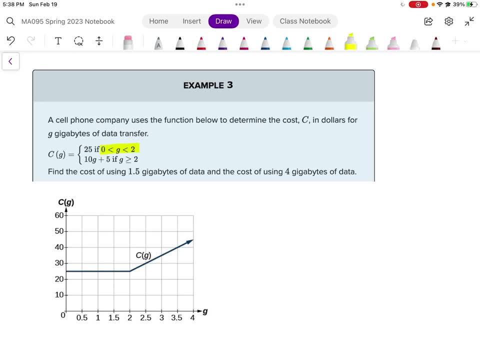 but greater than zero and less than two, your cost is going to be $25.. If you use greater than or equal to two gigabytes, your equation is going to be that one. So let me use two different colors there. So if it's greater than or equal to two, you're going to have 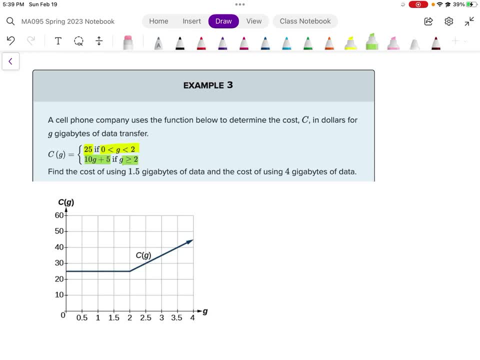 you're going to pay 10 times the number of gigabytes, plus five That will be your cost. So the question is: find the cost of using 1.5 gigabytes of data and the cost of using four. So pause the video and try that. 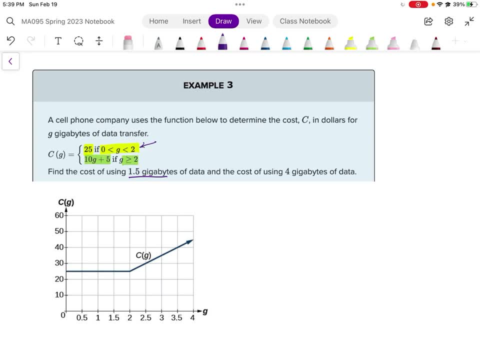 All right, so 1.5 gigabytes is going to be this, one here between zero and two. So the cost of 1.5 gigabytes is going to be $25.. Now the cost of four, the cost of four gigabytes, is going to be 10g plus five. 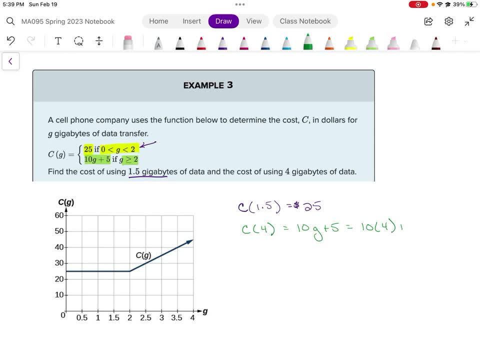 My g is four. so 10 times four plus five, That is $45.. Does that go with the graph? So find 1.5, and I'm right here, and that is still at $25.. Then find four, and that is over here, and that is at $45.. 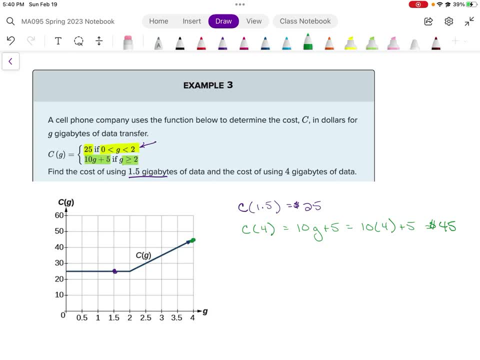 So that's $45.. That's $45.. That's $45.. Okay, so that is the graph of a piecewise function. That's what it looks like. So now people are going to be tempted when you graph these functions. 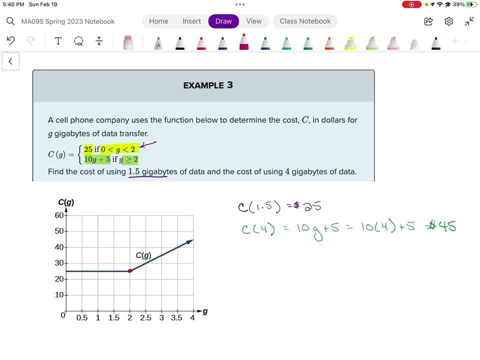 to put a point right here. You don't put a point in the middle. You don't put a point in the middle, Lumen will count it wrong if you're using Lumen or any online math program, because that is technically not correct to have a point in the middle. 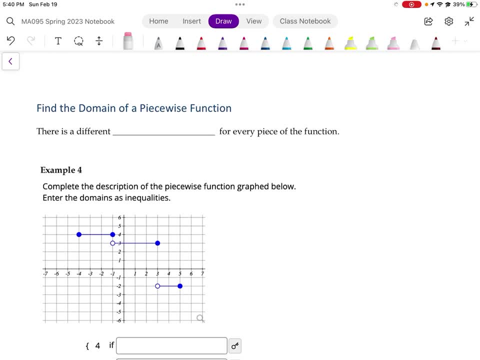 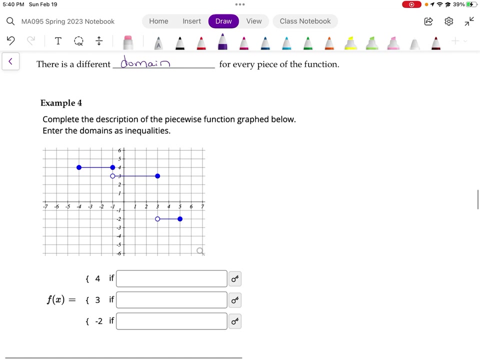 All right, so find the domain of a piecewise function. So remember there is a different, a different domain for every piece of the function. That's where piecewise comes from. Every piece of the function has a different domain. So this is the kind of problem you may see in the homework. 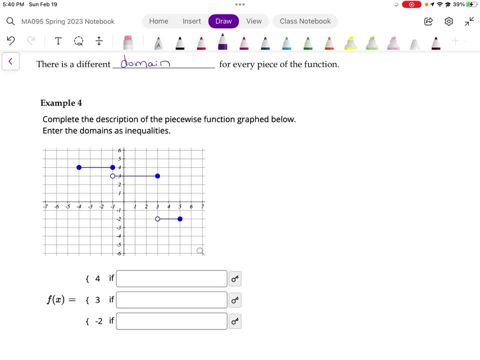 You're given a graph of a function and we are supposed to enter the domain as inequalities. Okay, so we're gonna use inequalities. So usually piecewise is written with inequalities, Not always All right. so f of x equals four. 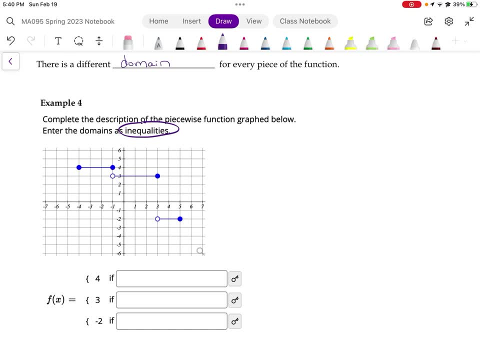 Which one is that? Well, f of x, remember. f of x is y. Y equals four. So where does y equal four? Well, it equals four right here, All right. so y equals four there. So what is the domain? 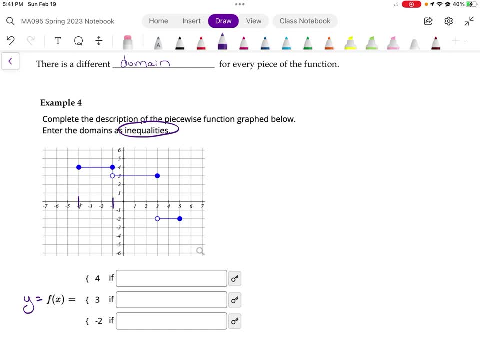 Well, it goes from negative four to negative one and it is solid so it includes them. So we're gonna say, if negative four is less than or equal to x is less than or equal to negative one, All right. so let's look at the next one. 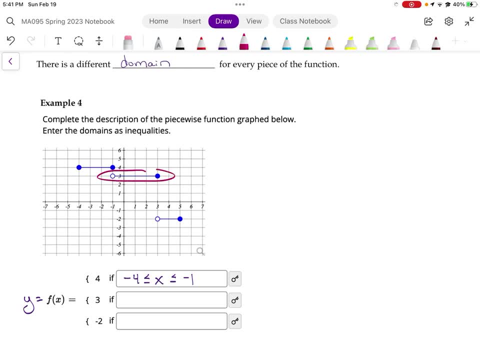 The next one is f of x or y equals three. That's that one, And that is gonna go between here negative one and here three. Now which one is open? Make sure you don't include that. So remember when it is an open circle. 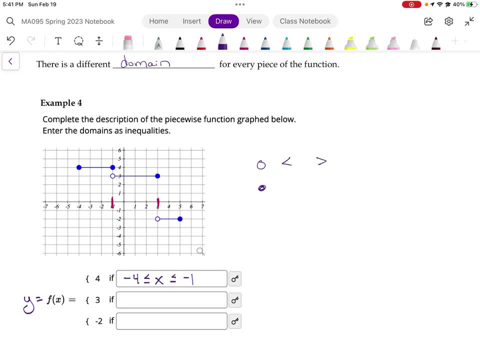 it's going to be those symbols. When it's a closed dot, it's gonna include the dot. So the open dot it literally means you're not including that point. So just think of it that way. The closed dot means this point is included. 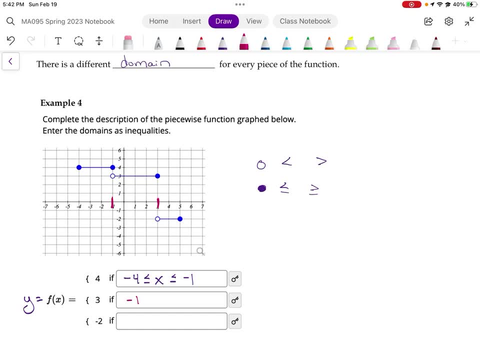 All right. so we've got from negative one is less than, x is less than or equal to three. All right, and that is because at negative one it's an open dot and at three it's closed. All right, you try the last one. 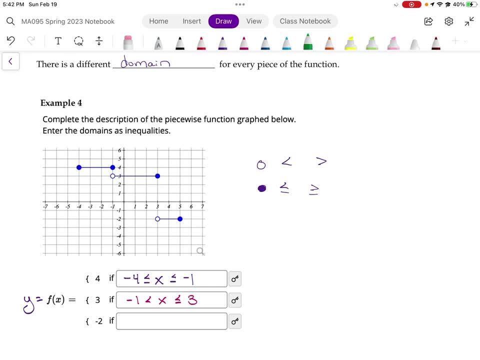 All right, here's our negative two, and it goes from three to five. It does not include three. So three is less than, x is less than or equal to five. All right. so question for you: What if that dot was closed in? 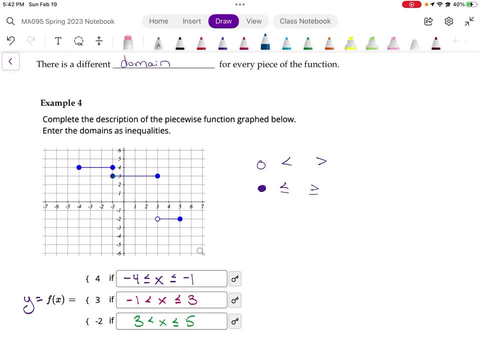 What is the problem with that? The problem is that it does not pass the vertical line test. This thing is no longer a function, because a vertical line goes through two points right there. So when you have a piecewise function, if it is a function. 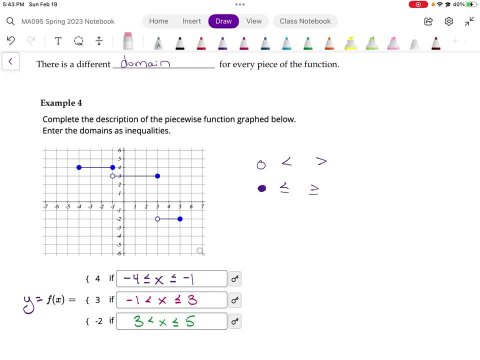 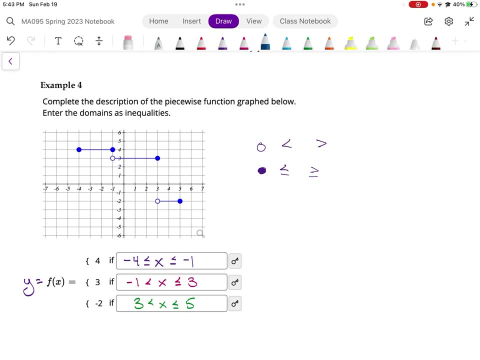 it can never have two dots, one above the other. So if I said what is f of negative one, What would you say, What is f of negative one from the graph? Well, you'd go to negative one right here and you'd find where the actual dot is. 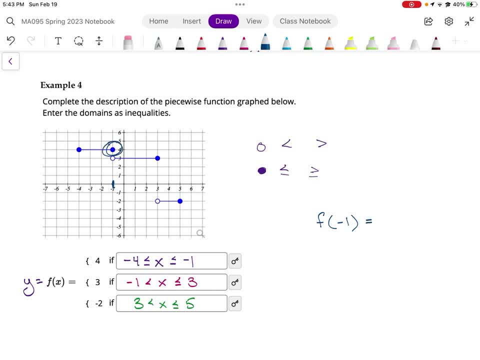 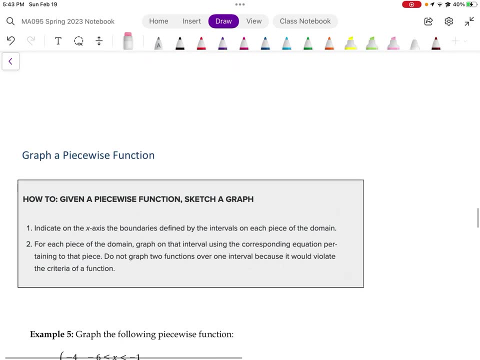 And it would be four. So f of negative one equals four. All right, so let's move on to the next question: Graphing a piecewise function. So now the steps are here. So the first step is to indicate the boundaries. 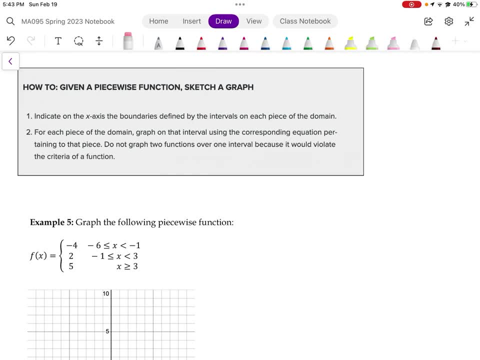 defined by the domain. You're not gonna graph those, but you just need to think about it. So I usually put it on my graph. somehow It's not gonna be on your final answer. So for each piece of the domain, graph on that interval using the corresponding equation. 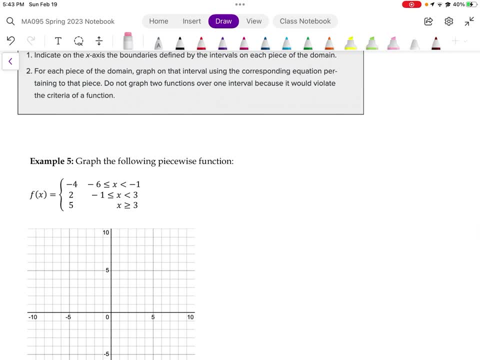 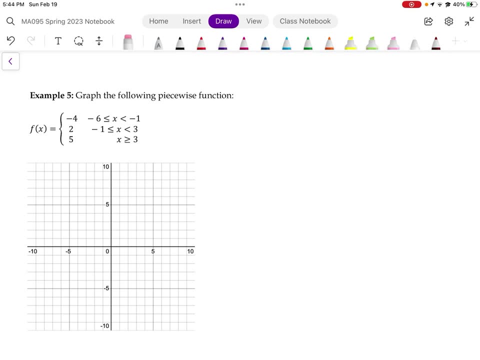 Do not graph two functions over one interval because it would violate being a function, like I was just saying above All, right, so f of x equals negative four. So this f of x equals negative four, that is just y equals negative four And it goes from: x equals negative six. 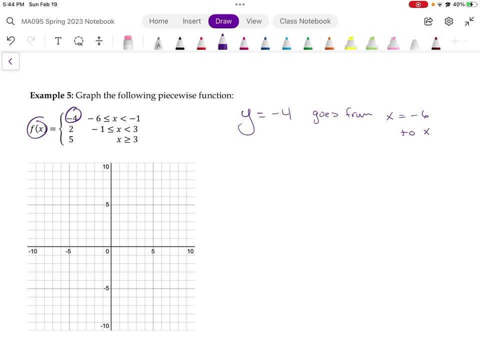 to x. not really equal six right right. not really equal to negative 1- I don't really know how to say that, I'm just trying to put it into English, but I'm looking at this domain right here. all right, so not really equal to negative 1, but it goes to the boundary. 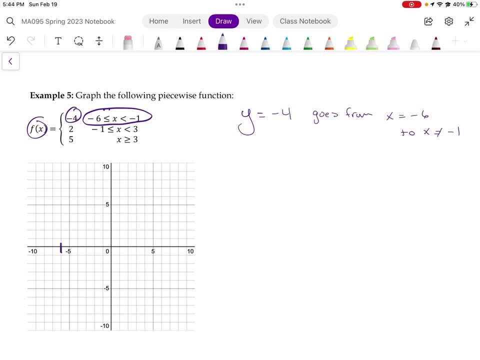 okay, so, from negative 6 to negative 1, but not including this one. right, we are going to have a line. y equals negative 4. well, what is this line right here? well, remember that's a horizontal line. horizontal line at y equals negative 4 and it goes from: let's see where's negative 4. negative 4 is here, so it goes. 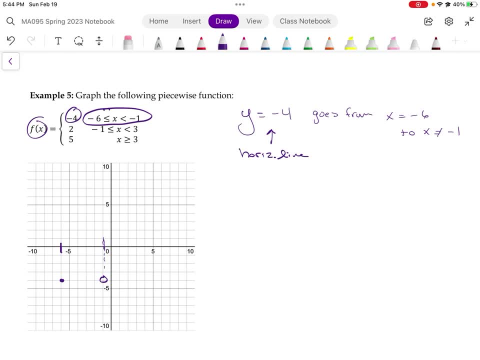 from here to here, all right. so from there to there, all right. so we're gonna put a line in between. so there's the first portion and I'm gonna erase all my mess that I made, all right. next, we've got y equals 2. y equals 2 when we're. 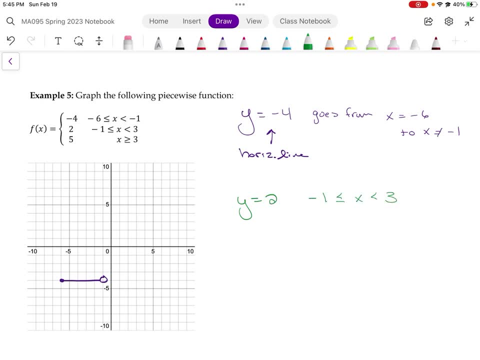 between negative 1 and 3. I'm gonna do it the right way. so remember: this means there's going to be a a, a, a closed dot here, and this means there's going to be an open dot. so at negative 1 there's going to be a closed dot and at 3 there's going to be an open dot and 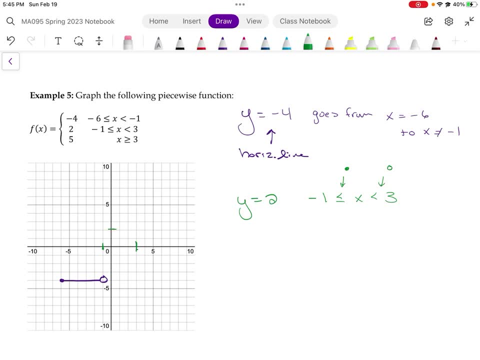 where is it going to be? well, it's going to be at y equals 2 here. so I've got closed dot, open dot and a line in between. that's the line y equals 2. okay, last one, do it in a bright color. it equals 5, y equals 5. 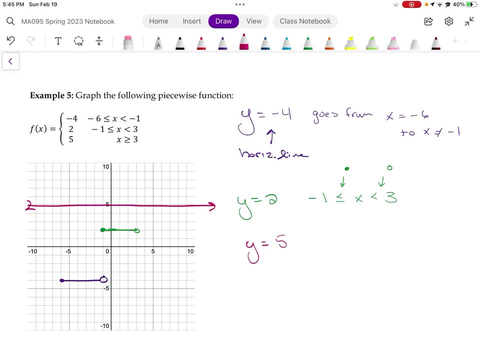 that's gonna be this line here, right, but it's only gonna go. it's only gonna go from X, from X is greater than or equal to 3. okay, so, when X is greater than or equal to 3. so remember that is going to be a closed dot. well, greater than or. 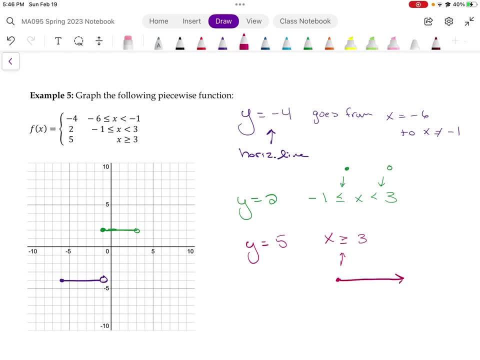 equal to means it's gonna go on forever. to the right, it's greater than, all right, so it starts. so let's see: y equals 5. that's right up here. this line here, so it starts at. X is greater than or equal to 3. okay, so this is considered a continuous. well, there's no real breaks in it, right? 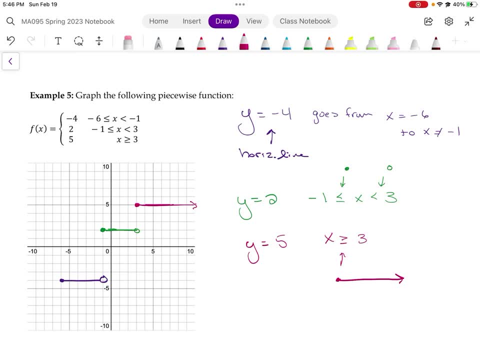 there's no open, there's no gaps between negative 4 and 2 to infinity, because if we get to negative 1, right, we choose one of them. well, we would choose this one. if we get to 3, we choose one of them, we choose that one. okay, I'm gonna erase. 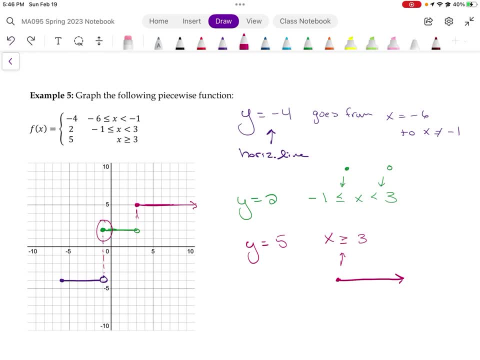 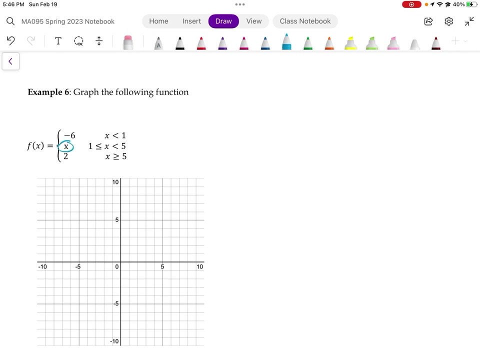 that, because don't you look back at it and think you need to write it down? okay, so that's how you graph a piecewise function. right now. here's a different kind. notice that the middle one is not just a horizontal line, so we're gonna have to think about that one. so let's do the two other parts first. so we've got y. 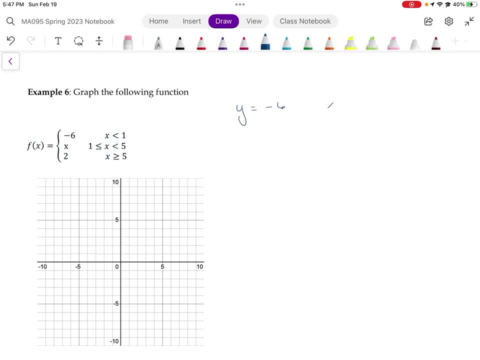 equals, or f of X equals negative 6 when X is less than 1. so it equals negative 6. so negative 6 is here, right, right there, and it's going to be from. X is less than 1. 1. 1. 1 is here, so there's an open circle, not not 5, 6, sorry, 6, all right, so there's an. 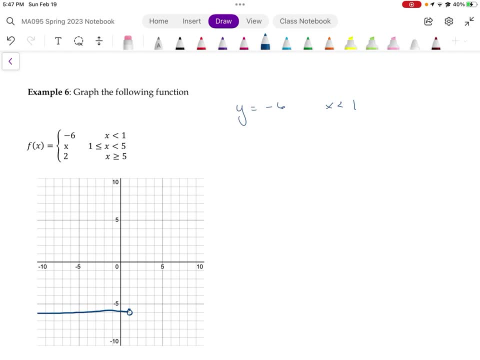 open circle at 1 and it's going to go all the way to the left right. that means all the way to infinity, remember? so if we did interval notation, we would say negative infinity to 1, not including 1. all right, so then I'm going to jump down. 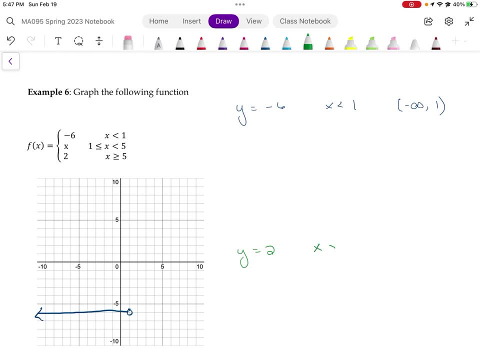 to the last one. y equals 2 when X is greater than or equal to 5, so that's going to be a closed circle. this one up here was an open circle, so greater than or equal to 5 means we're going to start here. there's our boundary and we're going to go to the right. okay so, and 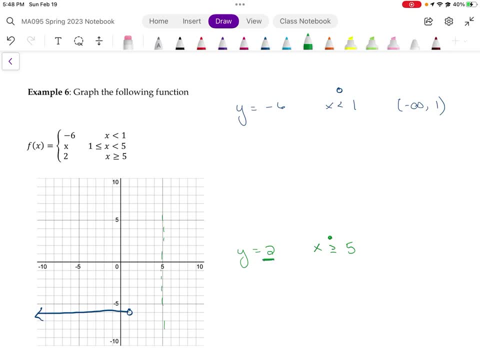 that is at y equals 2. so that's right here. so close dot, lots to think about, and off to the right. so many things to think about. I think I got it all right. so the last one, the last one is going to be this one here. so that is y equals X. 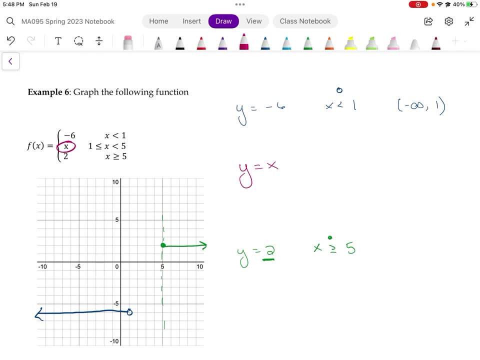 well, what does that look like? well, that looks like, you know, 1, 1, 2, 2, 3, 3, it's this line. here it goes directly horizontal. I mean sorry, directly diagonal, but it only goes from from here to here. it goes from 1 to 5. okay, 1 is less than or equal to, X is less than 5. 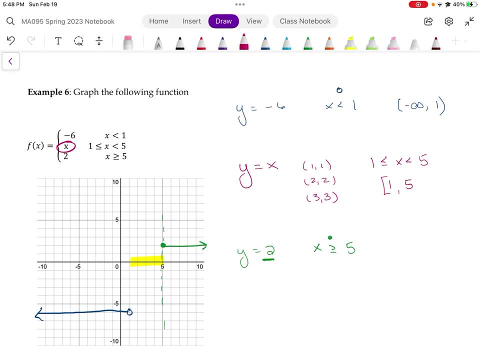 in other words, it goes from 1 to 5, like that. so this one is going to be a closed circle and it's going to be a closed circle. this one is going to be a closed dot and this one is going to be open, but where? 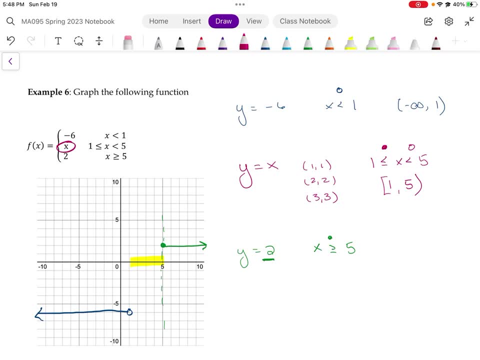 do you start? well, at 1. it needs to start at 1. so 1, 1, right, 1, 1. and then we go to and that's a closed dot. and then we go to 2, 2, 3, 3, 4, 4, and then, when we get to, 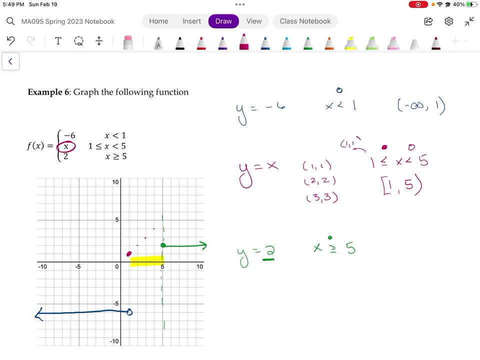 5. this end right here. so this end is 1: 1. this end is 5: 5, but it's an open dot, so 5: 5 is 6 here. now we have to just fill in in between straight line, and that's how you. 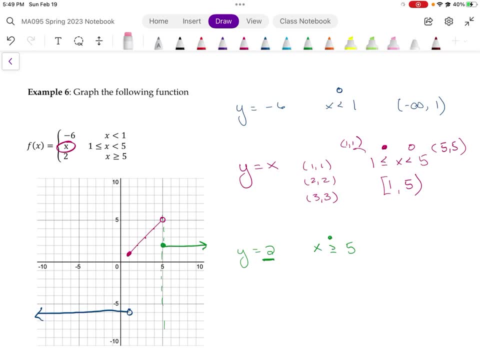 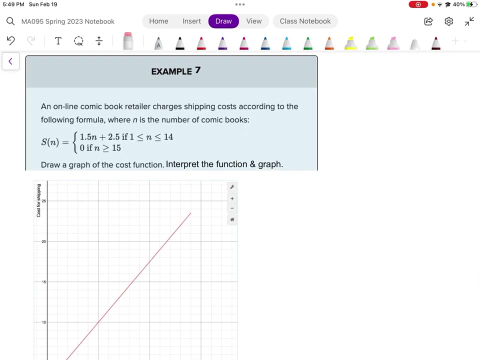 do it. yes, you just find what the line looks like in the space and you won't have any much harder lines in this class than just X or maybe 2x or something like that. all right, let's look at a couple more examples. this is a real-life. 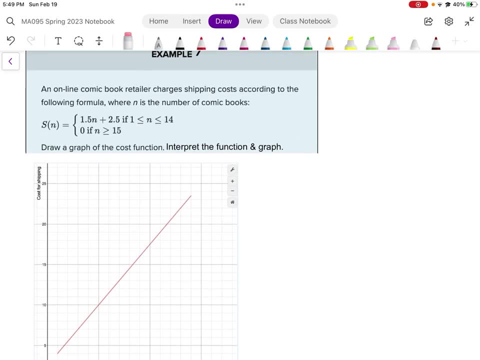 situation. we're just gonna look at this one. an online comic book real estate retailer charges shipping costs according to the following formula: where n is the number of comic books, n is the number of comic books that a person buys. so if they buy between 1 and 14, 1 to 14, this is the 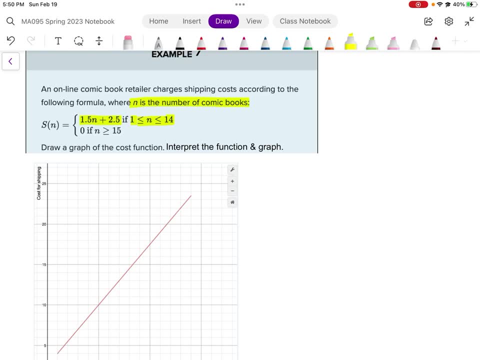 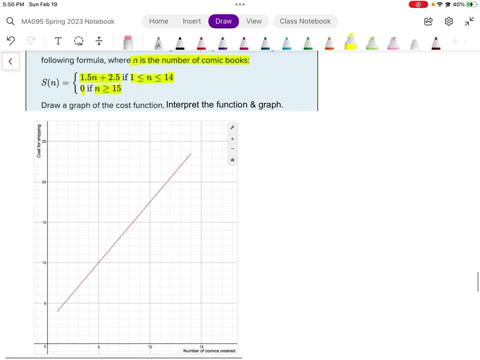 shipping cost. if they sell fit, if they buy 15 or more, they don't have to pay shipping. it's free, all right. so this line must then start at 1, because anything less than that doesn't make sense. you can't, you don't buy zero, you. 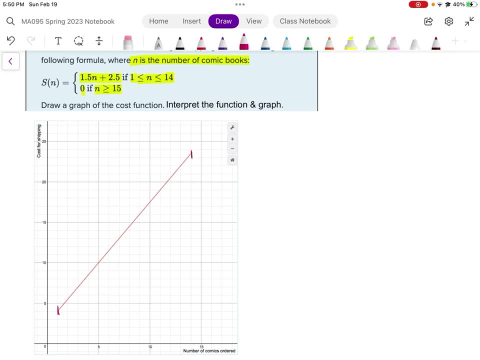 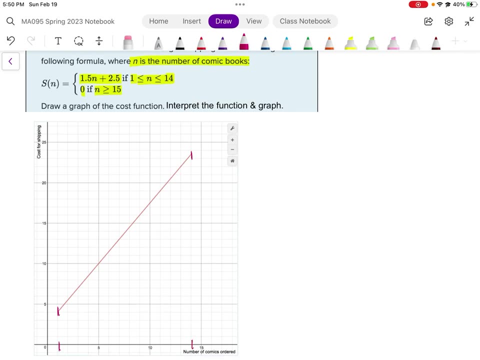 don't buy zero comic books. and then up to 14. so this thing goes from 1 up to 14. well then, how are you going to say: s of n equals 0 at 15 or more? well, that line would be from here on forever. so here we. 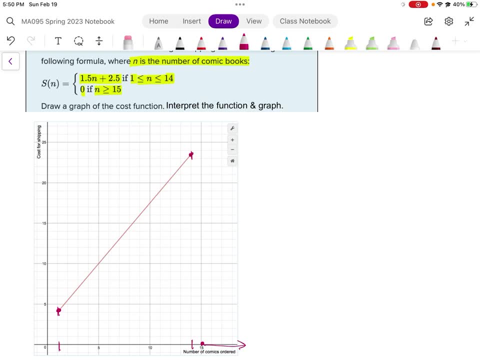 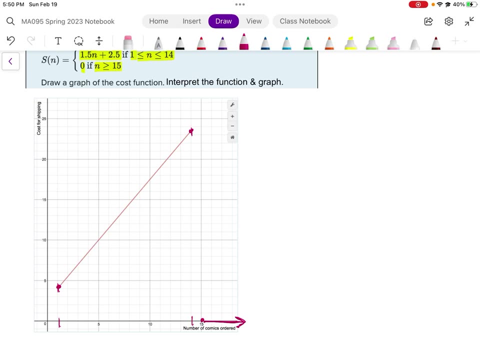 should have a dot at the end and a closed dot at the end, and then the last line would be what I drew at the bottom, maybe a little straighter than that, but like that all right. so that means if I saw, if I bought 10 comic books, my cost. 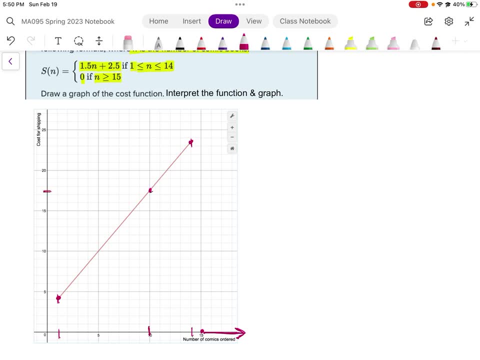 would be right here around 1750. if I bought 5 comic books, my shipping would be $10. so if I bought 15 or 16 or 17, I wouldn't have to pay any shipping. so that's how that's a piecewise function in the real world. all right, so I'm gonna. 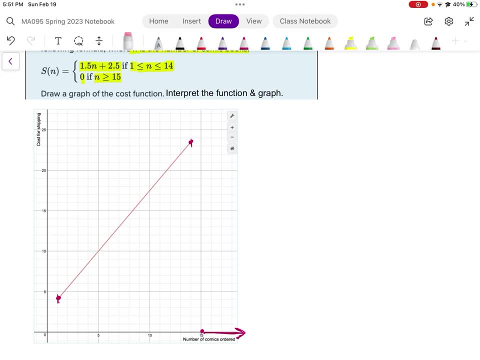 erase some of those. okay. identify the domain and range of a continuous piecewise function. we've done some things like this, but this is what it looks like for a continuous piecewise function. that such as showing that's a смыс. it does things like that, but this is what it looks like for a 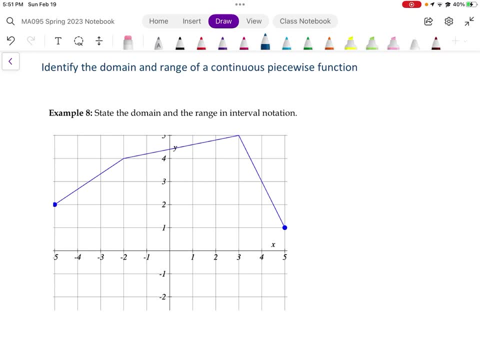 continuous, piecewise function. Notice, there's no breaks. Continuous means you would never, you don't pick up your pencil, You would just draw, draw, draw and you would never pick up your pencil. okay, So the domain of this is going to go from. 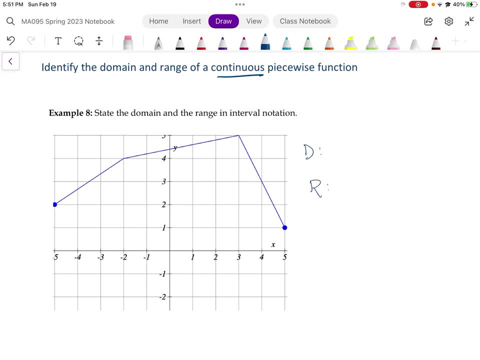 the very left to the very right and the range from the very bottom to the top. So pause the video and see if you can get the domain and range correct. Okay, so the domain goes from negative five to five and it includes them because it has a